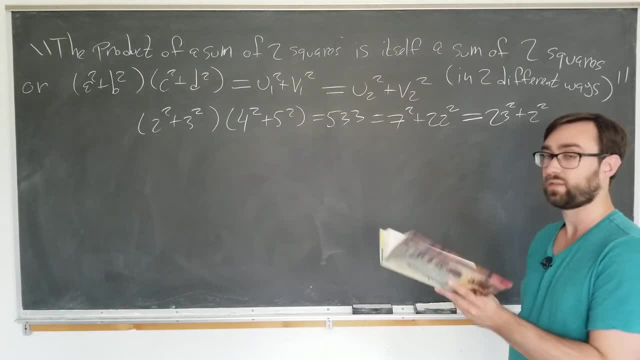 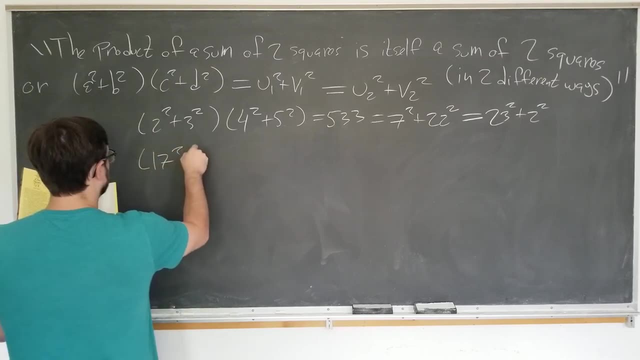 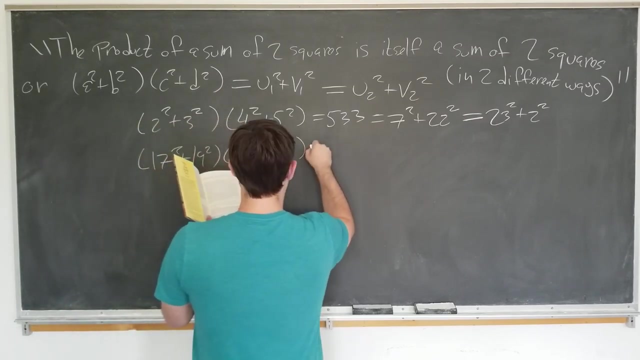 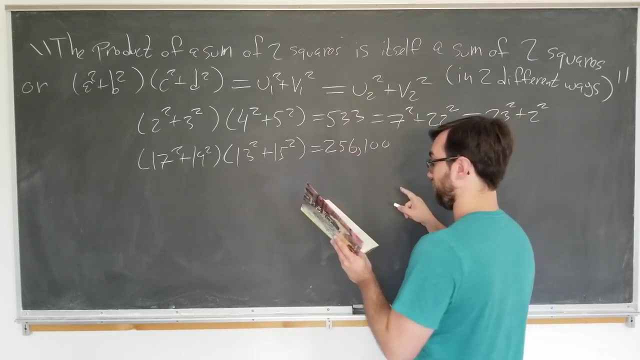 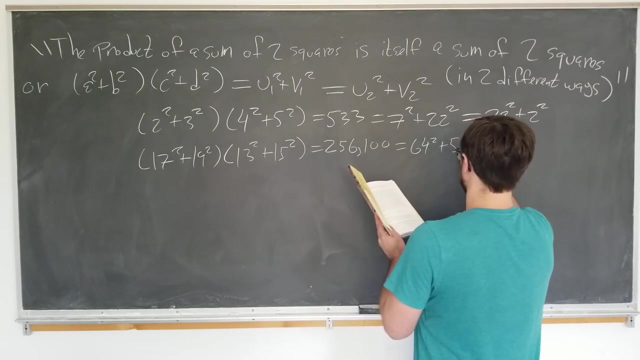 smallest examples. There are other larger examples as well, which you can also verify, So I'm going to verify. Second example given in the book is that 17 squared plus 19 squared times 13 squared plus 15 squared is equal to 2,500.no 256,100, which we can also write as 64 squared plus 502 squared. Wow, 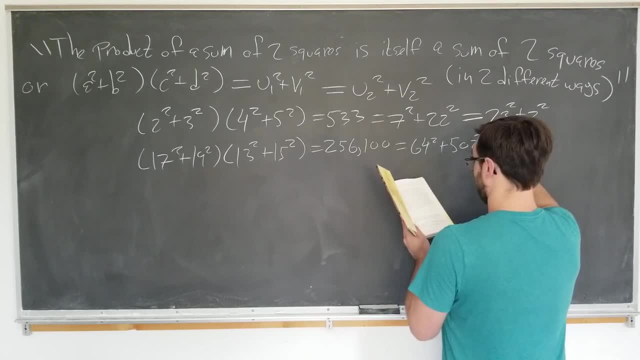 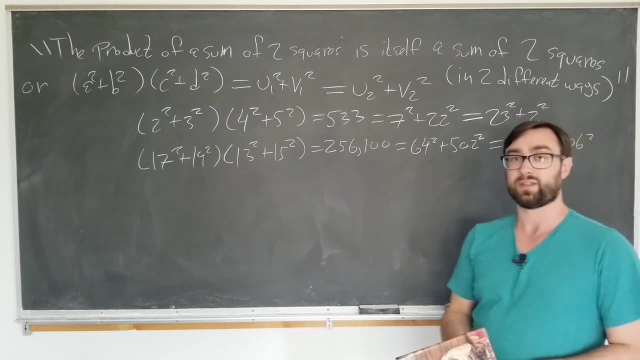 there's just so many numbers right, Way more numbers than I'm used to. You can also write as: 8 squared plus 506 squared. You can, of course, feel free to verify these. Just a lot of numbers, though. There's a lot of patterns that you. 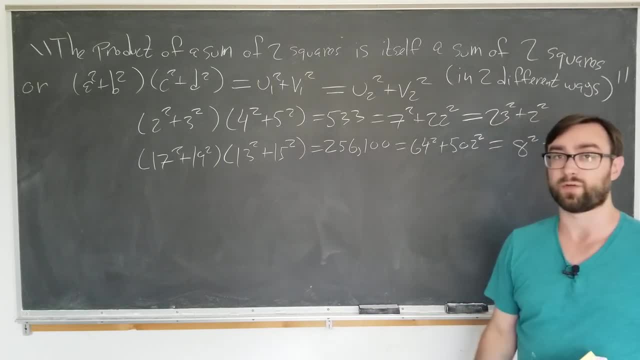 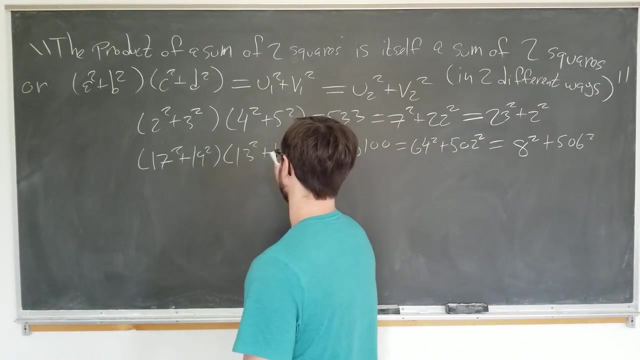 can discover just by plugging numbers into your calculator and so forth. I'm not sure if this is the way how these were originally were discovered, But let's say that we suspected that this pattern holds for any A, B, C and D, So any number that we put here should be equal to the number that we 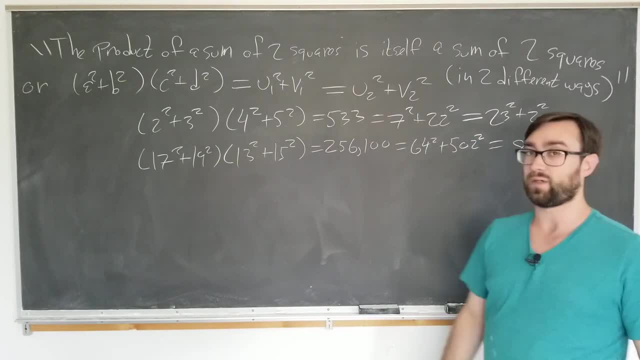 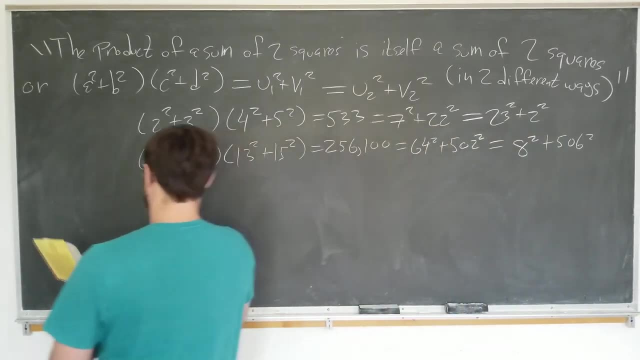 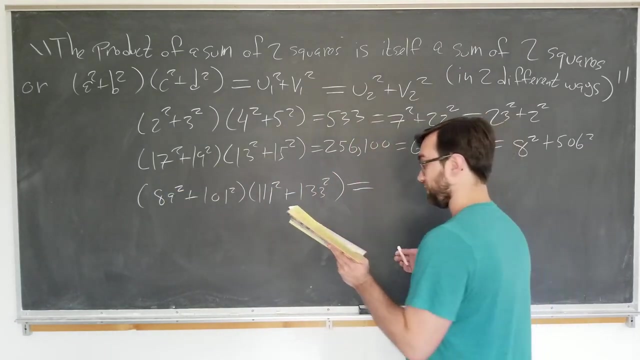 know. So how are we going to go about finding that? Let's say, as the book indicates to us, that we're going to begin with the following example: 89 squared plus 101 squared. I'll multiply it by 111 squared plus 133 squared. This is a huge number. if we multiply this out, This is 543,841,240.. 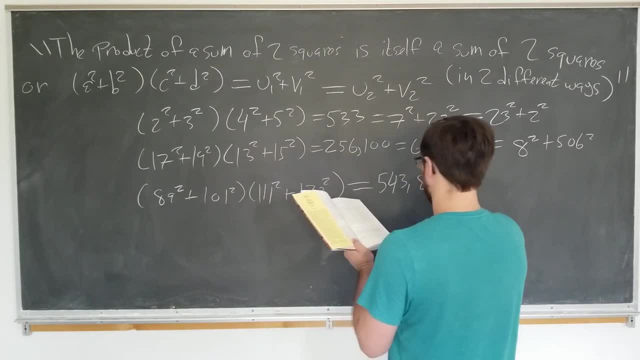 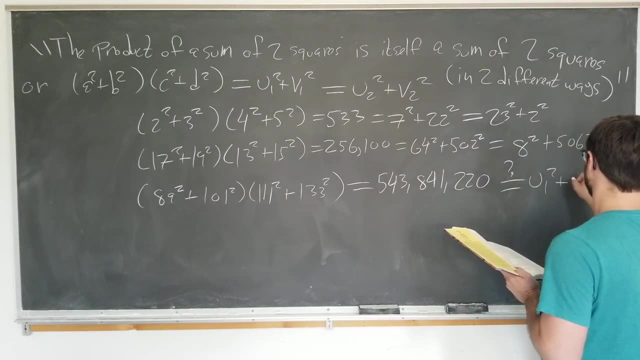 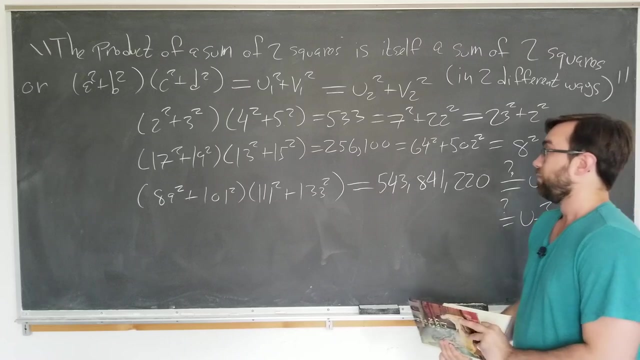 So this is a huge number. if we multiply this out, This is 543,841,240.. And we want to express this as some u1 squared plus v1 squared and u2 squared plus v2 squared. We're assuming that we found the other two simply by brute force calculation And we wanted to. 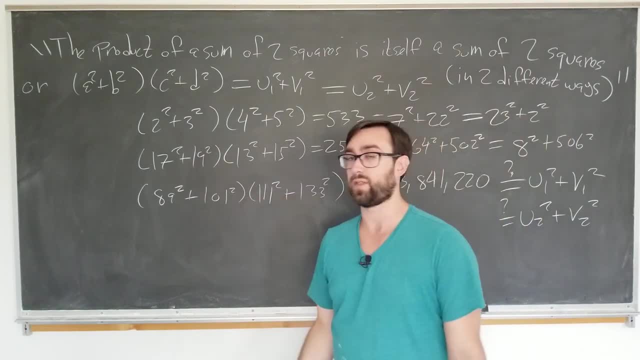 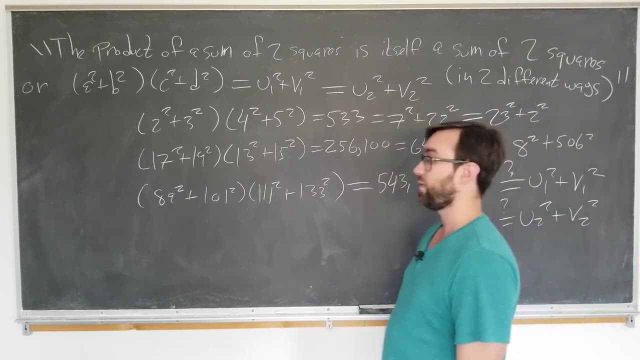 generalize it to these random numbers, because we think it should hold true for any numbers. The question is: how do we find u1,, v1,, u2, and v2? Well, there are apparently ways to do this: using Diophantine equations. 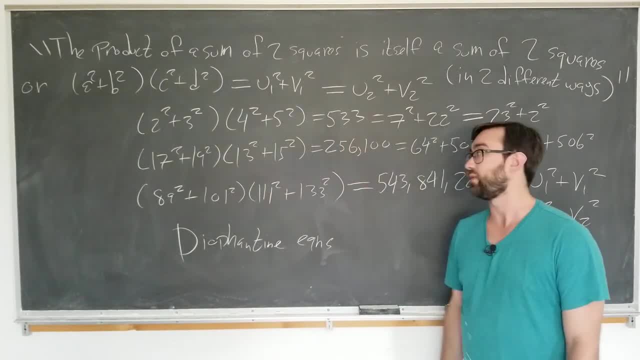 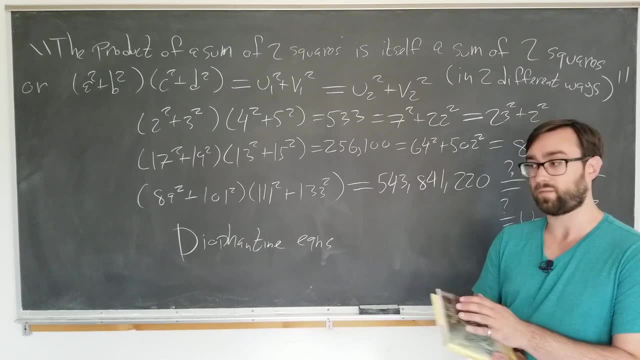 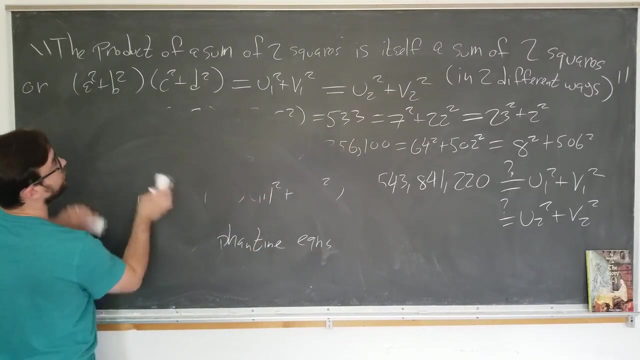 which we're not going to cover here. I find them to be quite boring, actually, But we are going to show this using a complex method. So, yeah, that is the setup. Let's get started with the proof. All right, Product of the sum of squares is itself a sum of squares. 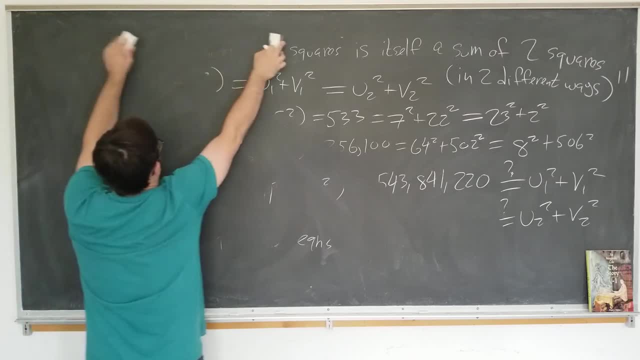 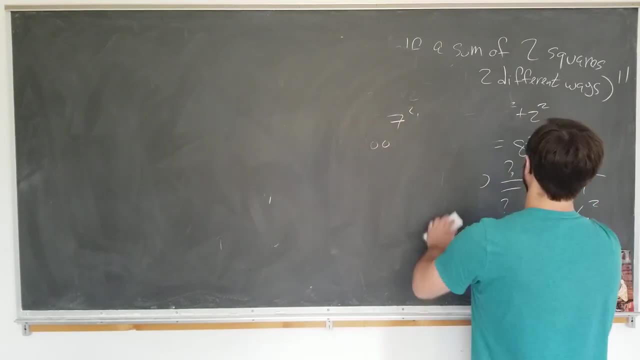 holds for two squares. of course It may hold for more, but we're not gonna cover that in this video. Maybe you can find out if it holds for more squares. I really don't know personally. I don't know if it holds for more squares, Okay. 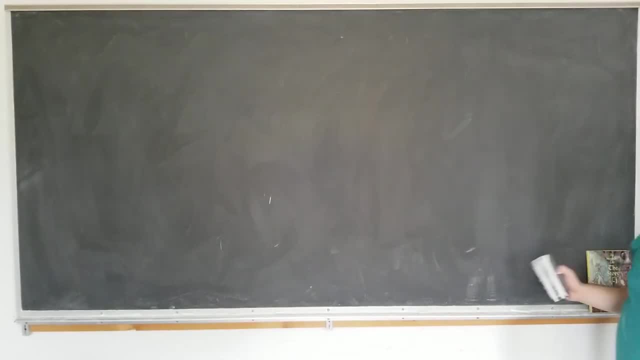 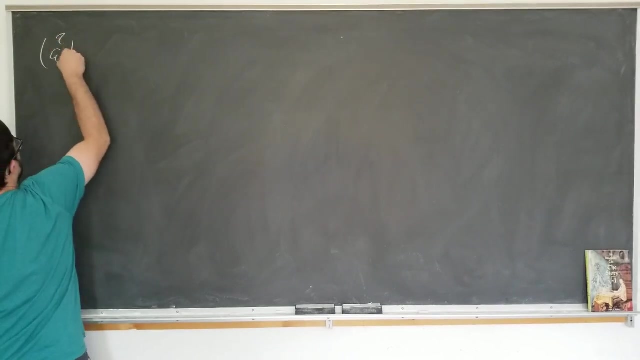 But definitely check out this book, Imaginary Tail. It's fantastic. It has great examples like this. Shows you the utility of complex numbers without even using calculus where they're really important. Okay, So we're gonna start with the left-hand side of our expression. We had a squared plus b squared times c. 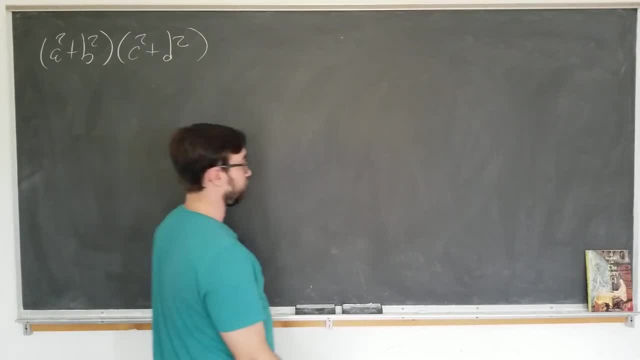 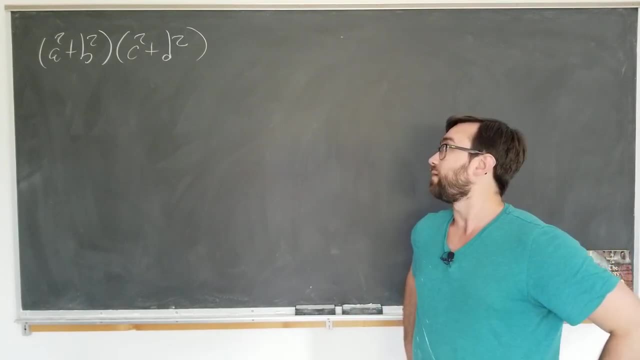 squared plus b squared. That's what we had before. Now I'll give you a hint that we're going to use complex numbers for this. So one thing you might think right off the bat is: this looks like a magnitude of a complex number. 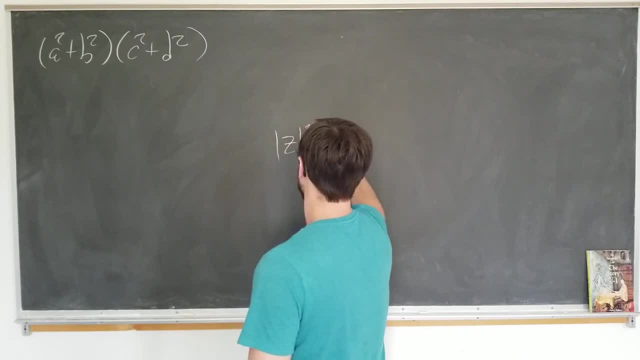 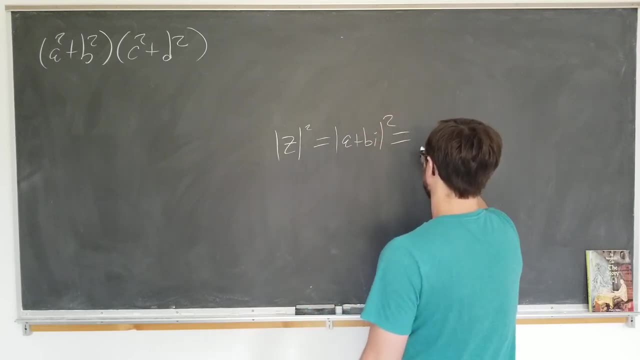 and since you know the formula, that absolute value of some complex number squared, but right in terms of a plus bi, is simply a squared plus b squared. So we can see right off the bat that, if we want to, we can recognize these two. 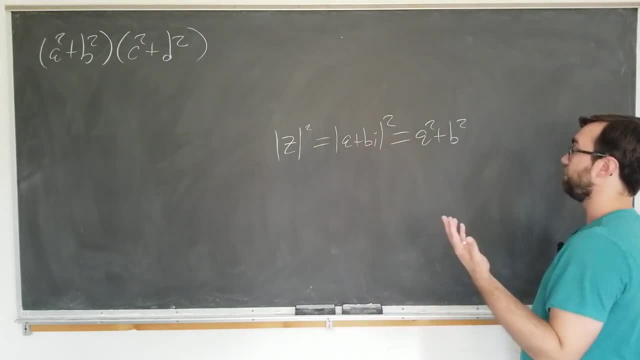 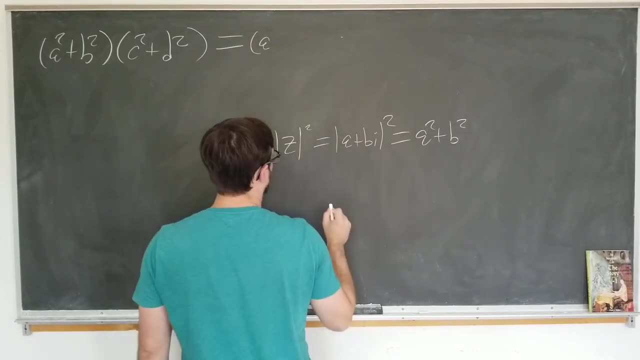 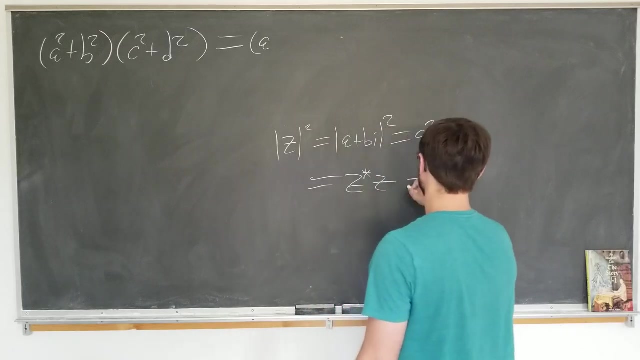 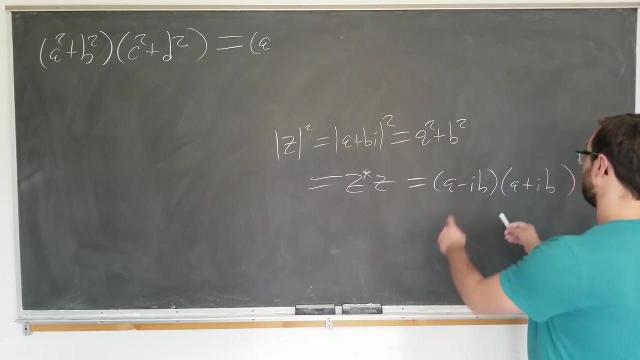 products is simply the magnitude of a complex number. Let's go ahead and do that for both of these here. So we're gonna use the following form: It's going to be equal to z, star z, or a minus i b, a plus i b. you can see this, since we have a squared. 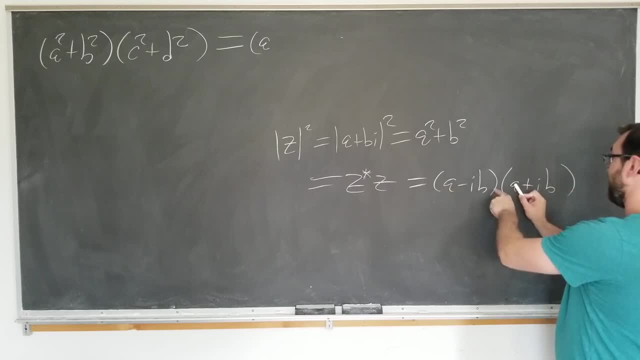 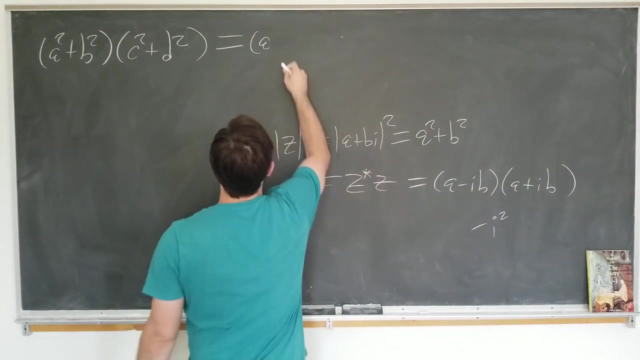 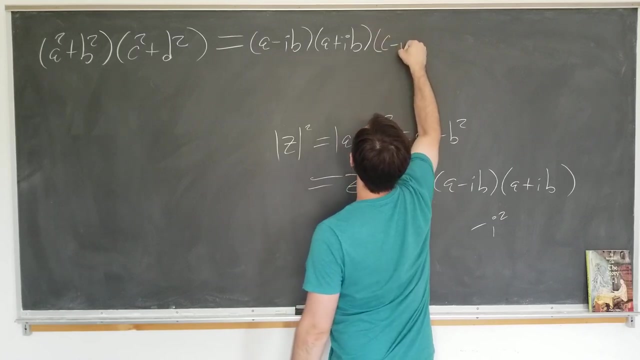 here we have i a b and minus i a b, which cancel out, and we have minus i squared times b, which which is, uh, one, of course. so which is a squared plus b squared? yep, so now we're going to write this as a minus i b, a plus i b. now we're going to have c minus i d, c plus i d. okay, now you see. 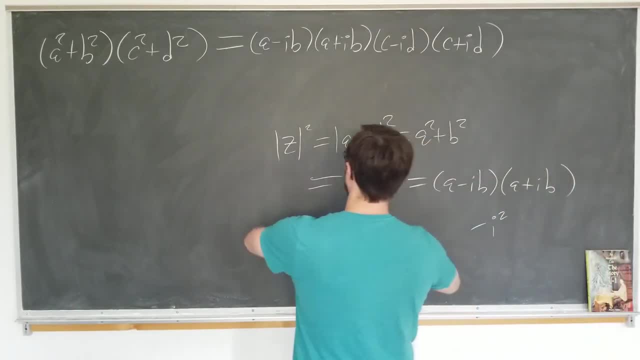 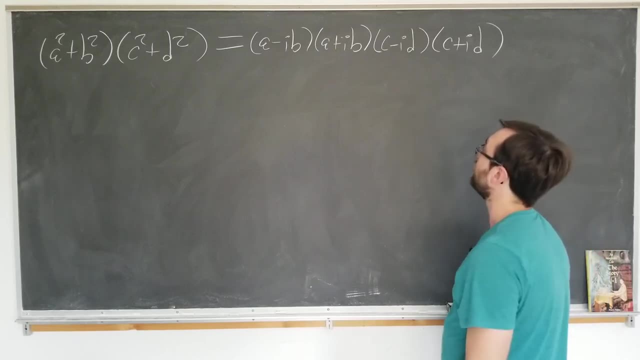 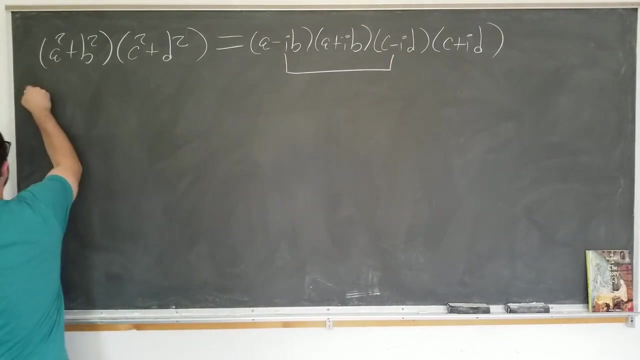 immediately that we have more structure to work with than we did before. all right, so first thing that we're going to do is multiply them in the following way: we're going to group these two, get these two together and multiply them. so if we do that, we have 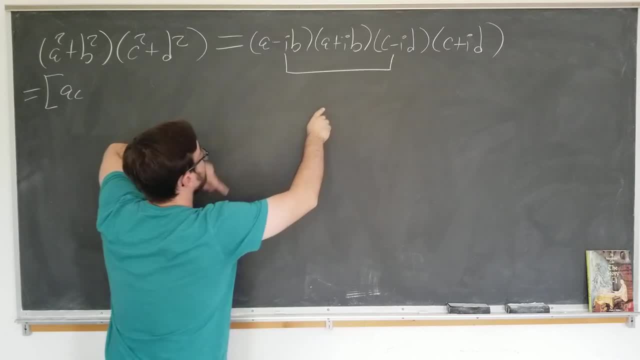 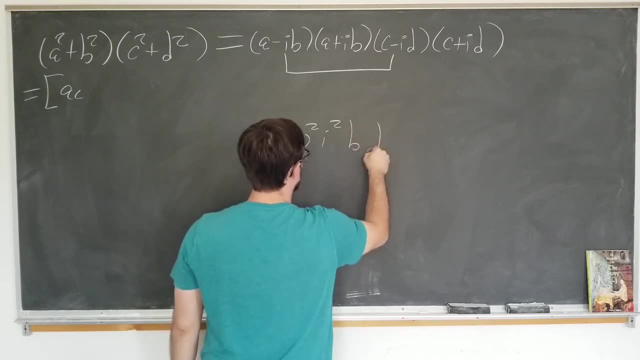 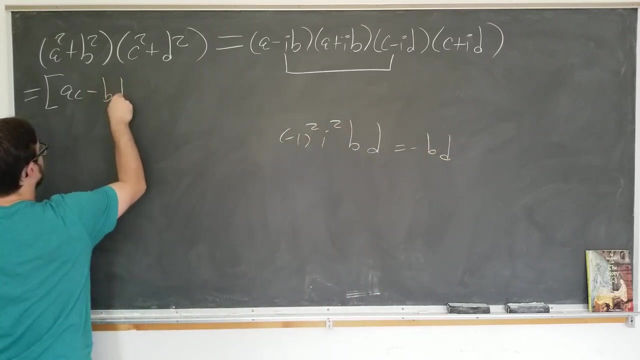 a c. the other real term is going to be the last term. so it's minus one squared i squared b d, which is obviously minus b d. gotta keep track of these signs here: a c minus b d. and we have an i term here. what is the i term? 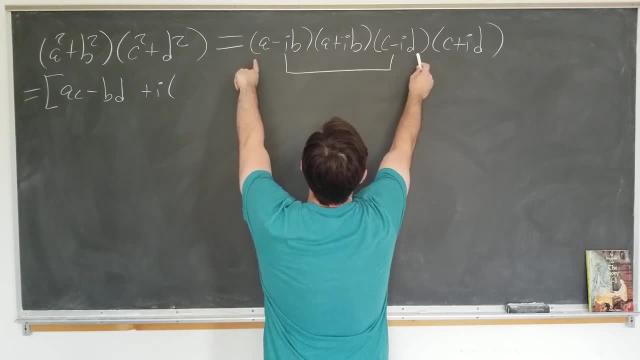 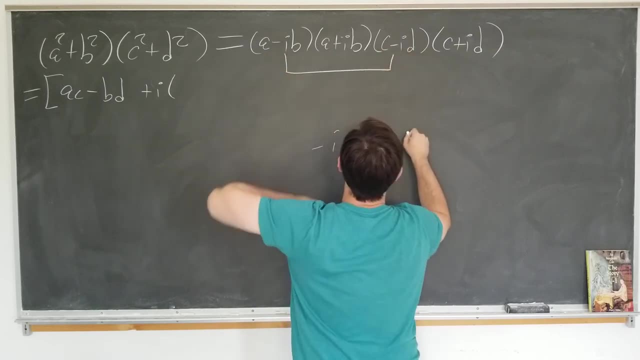 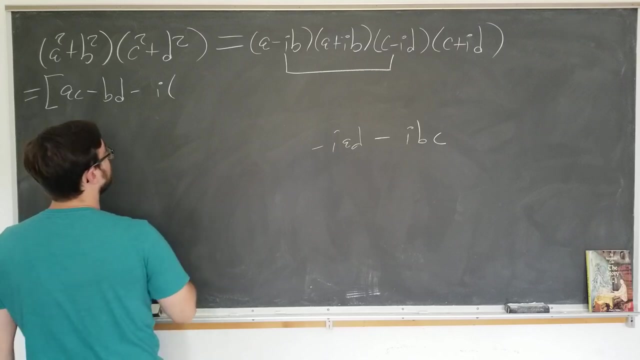 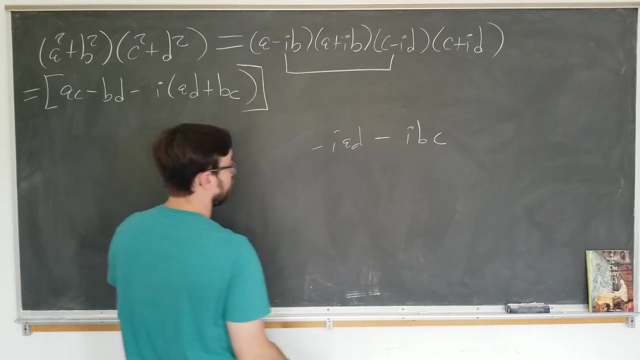 a c. we have minus i a d. we also have minus i b c, so we're going to actually write it in this form: i have minus. i times the sum of these a d plus b c. fantastic. and now what we're going to do is multiply. yeah. 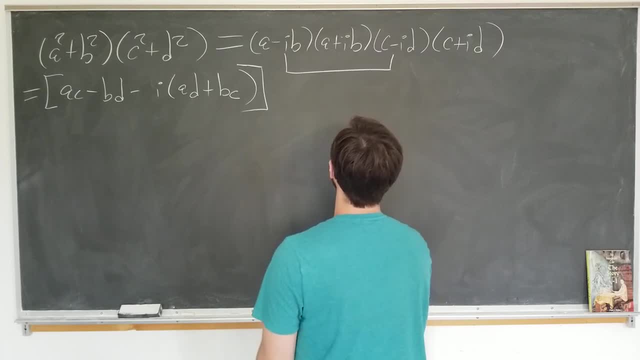 i'm going to keep that there for reference. we're running out of room, though. multiply the other two together. so we did the first two. now we're going to do the last two. multiply these bad boys together, all right? so if we do that, we have a- c, and the other real term is i squared b- d, so it's minus. 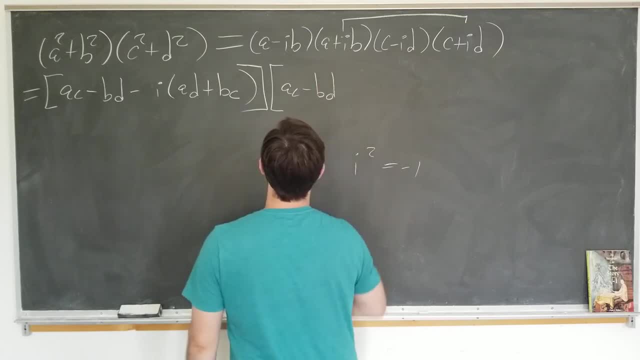 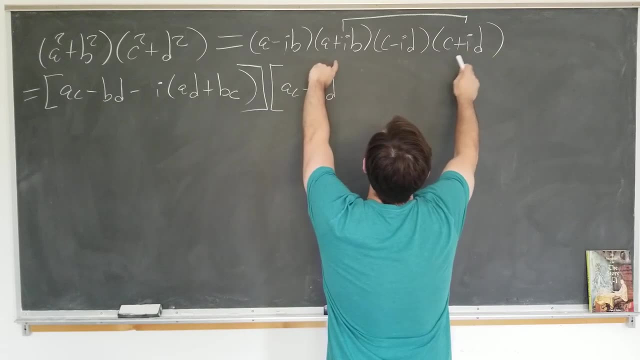 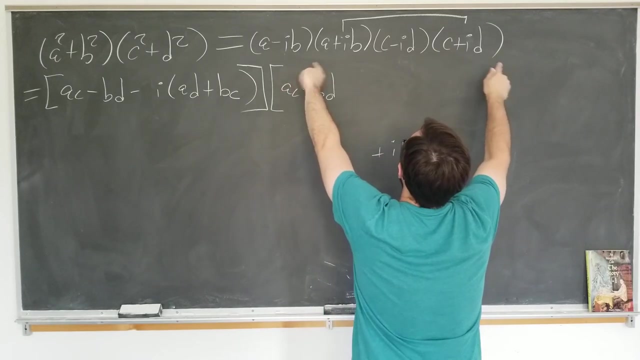 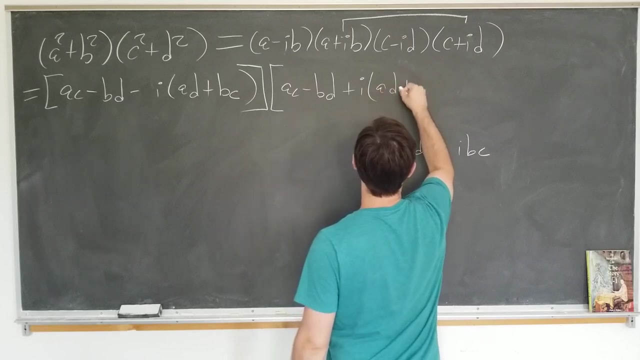 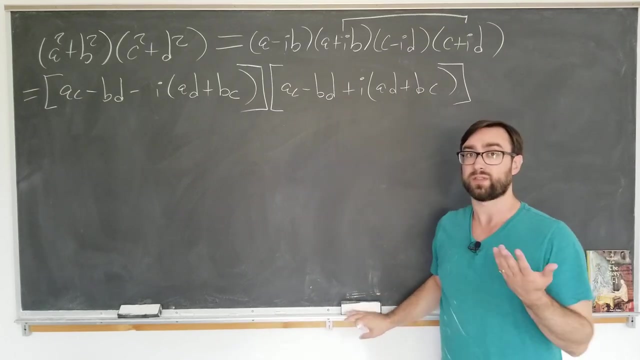 minus b d sounds good and the imaginary term um. so we have plus i a d, plus i b c, so it's plus i what we had before. now, looking at this, we notice something quite remarkable. it's actually not remarkable for a reason, i'll explain later, but something that 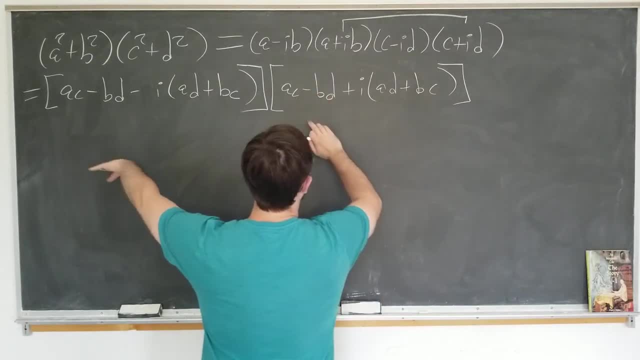 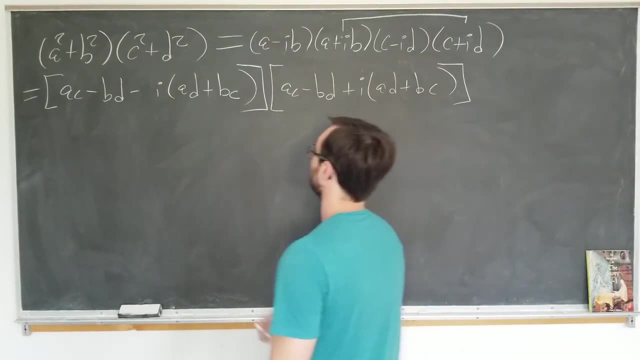 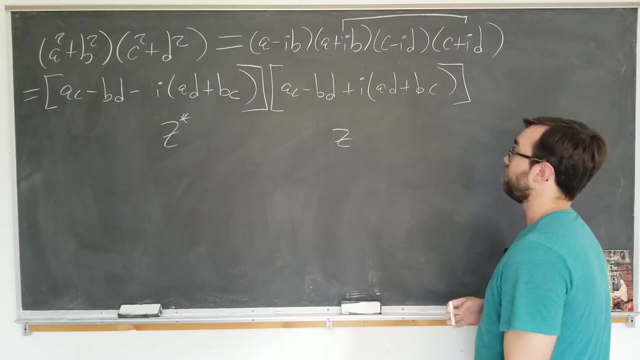 absolutely appears remarkable. so we have the same real component, but the imaginary component is the same, but separated by a minus i, so it's conjugate. so this is a form of you know, z star, z by itself, which we can now write as a squared plus b squared. but these are not the normal a's and b's, these are 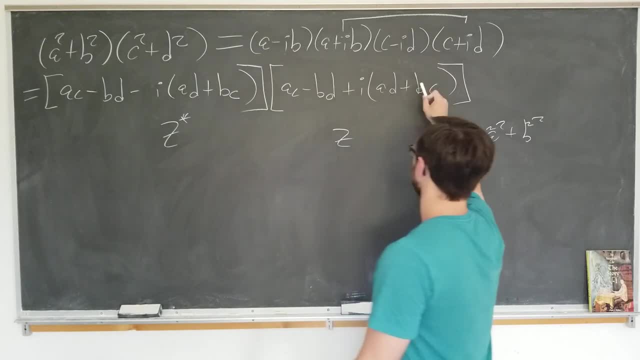 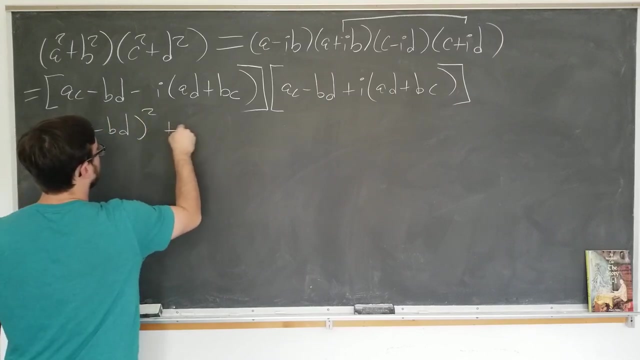 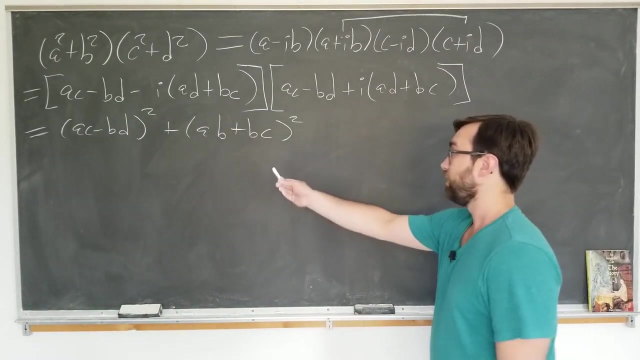 this being a and this being b. so we can immediately write this down without actually multiplying out all the terms. this is simply a c minus b d squared, plus a d plus b c squared. so actually we have the first solution, we have the first u1 and v1 here. now i want to take this time and note that if i gave this 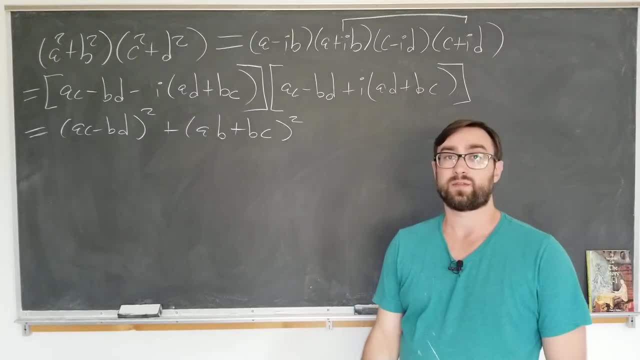 to you in an exam or something. i'm going to write this down, and i'm going to write this down in a different way, and i'm going to write this down in a different way, and i'm going to write this down in a different way, and i just wanted you to show that it was true. you could easily foil both of these terms and show 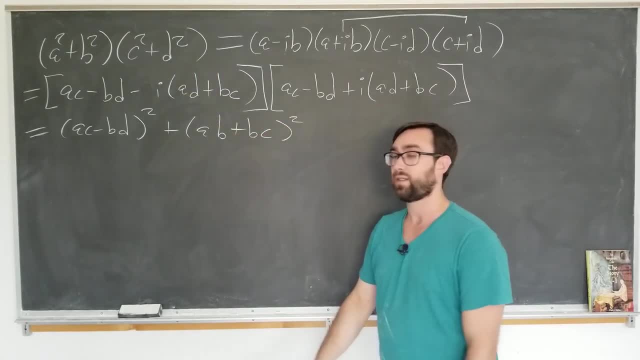 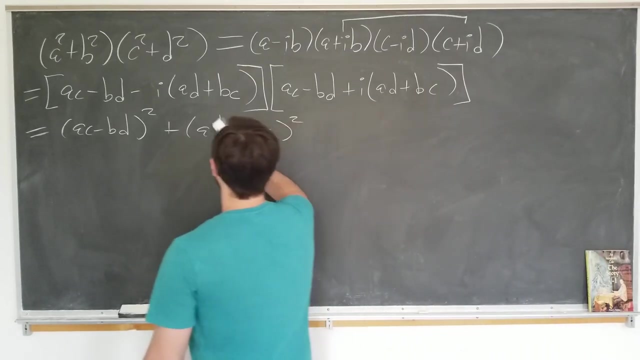 that it is indeed equal to the product that we have up there, but that's not very illuminating. you wouldn't actually learn anything by doing that, and in fact, that's not how this relation was described originally. i mean, how would you come up with this? how would you come up with this? 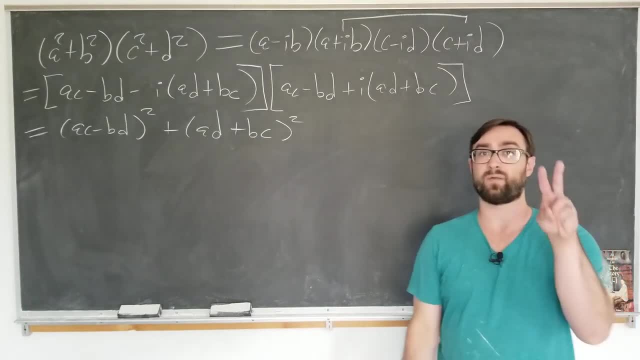 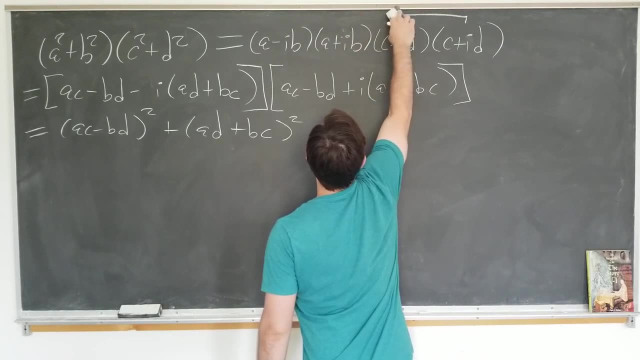 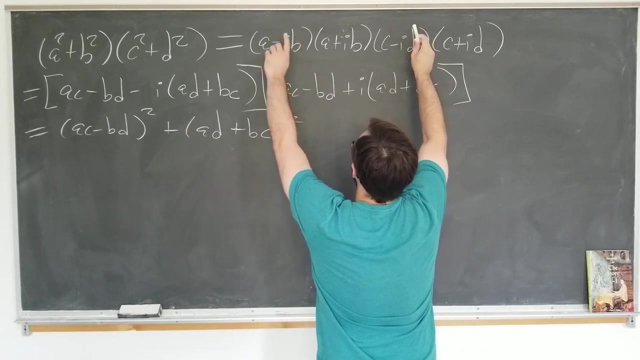 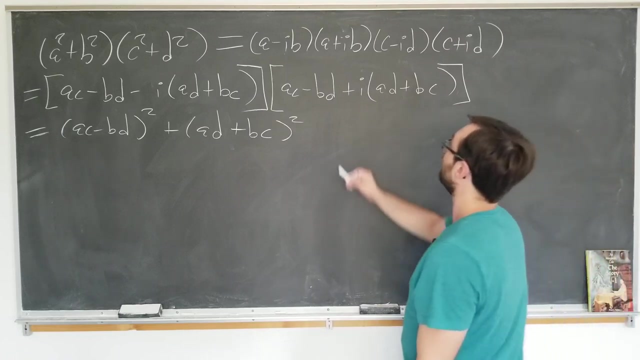 originally okay, so let's find the second one. i told you there were two solutions. i only found one. all right, so how are we going to do this? well, it's pretty straightforward. so last time we multiplied this one and this one. but we don't have to do that, we can go the other way. so we did the first and the last terms of the product. 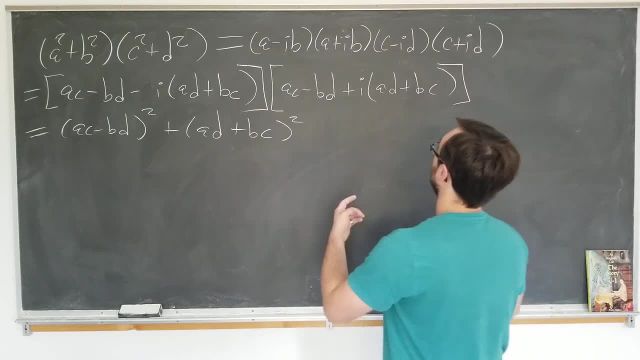 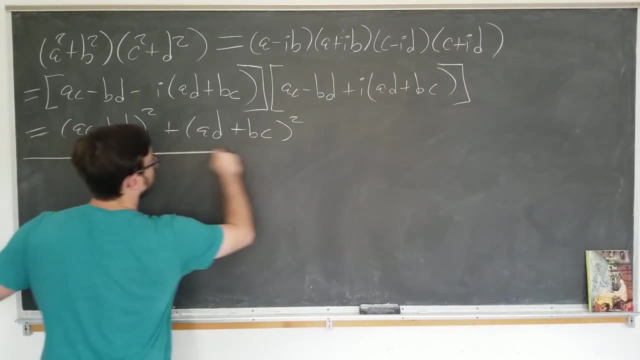 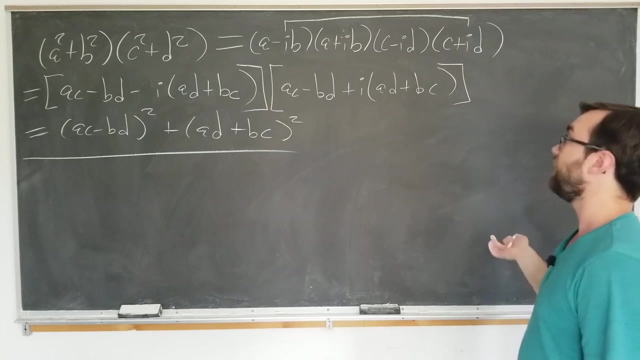 if we use the foil method terms. but we don't have to do that. we can multiply the outer and the inner terms. so So let's go get and get our second solution. by doing that, We are now multiplying these terms together. Note, we did not do that before. 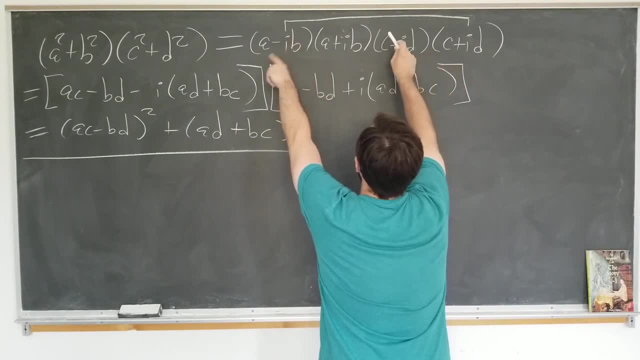 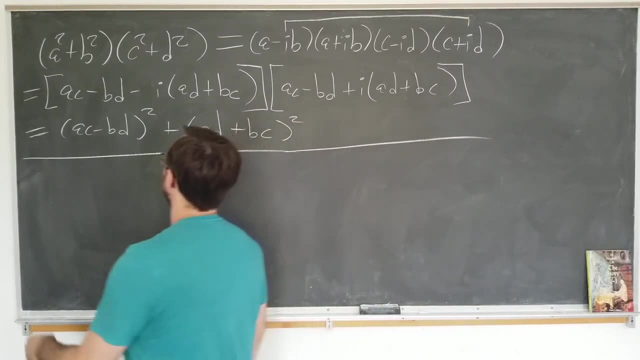 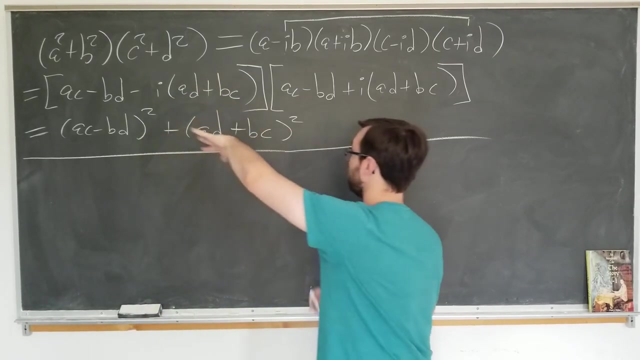 We multiplied the outer and the first and the last. Now we're going to multiply the outer and the inner terms together. All right, Lot of kind of tedious multiplication here, but because of the ZZ star simplification, there's only one step of tedium, so it's worth it. 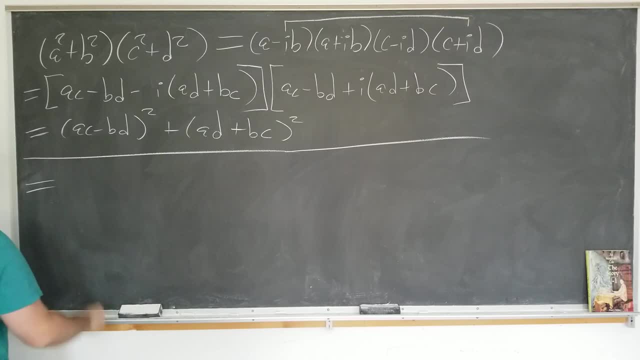 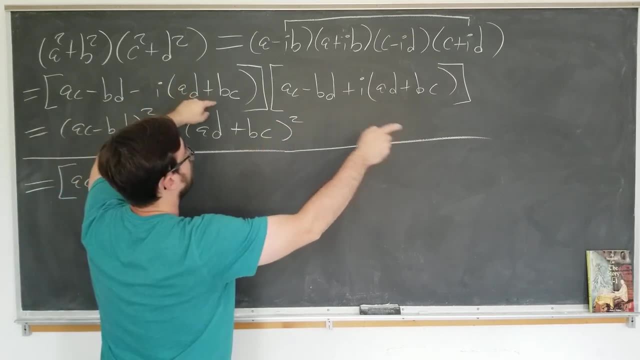 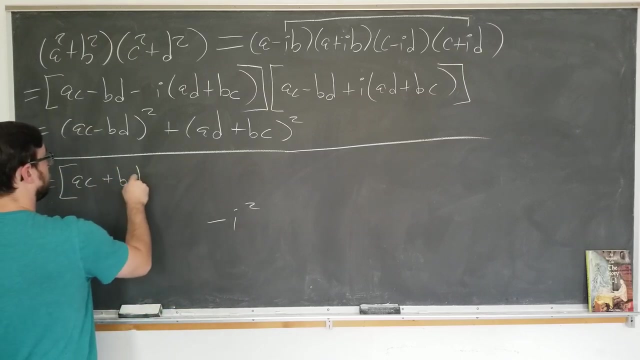 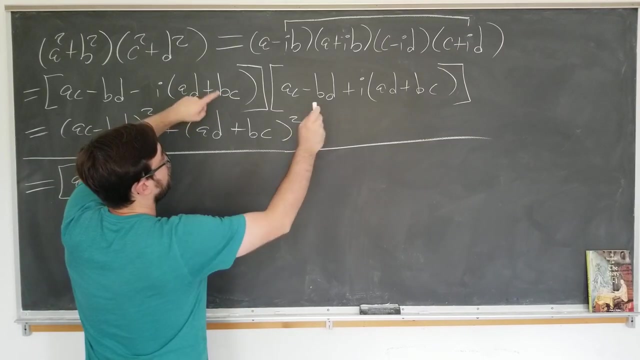 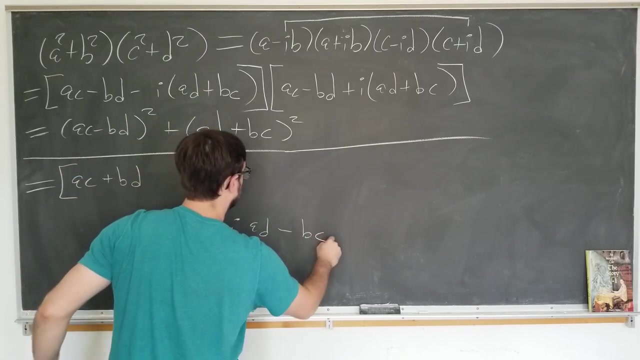 Okay, This is also equal to. We have AC. Last term is minus, I squared BD, So that becomes plus And the imaginary term is AC, IAD minus BC, And we want to use the same format that we had over there. 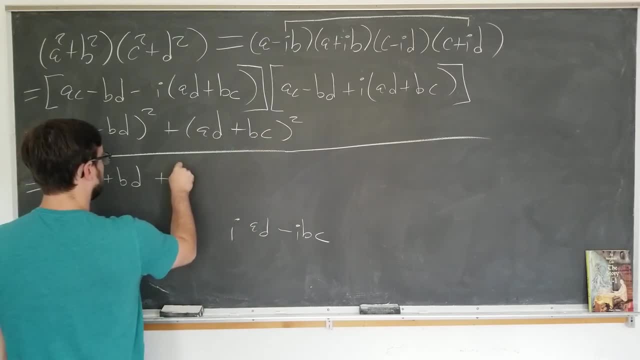 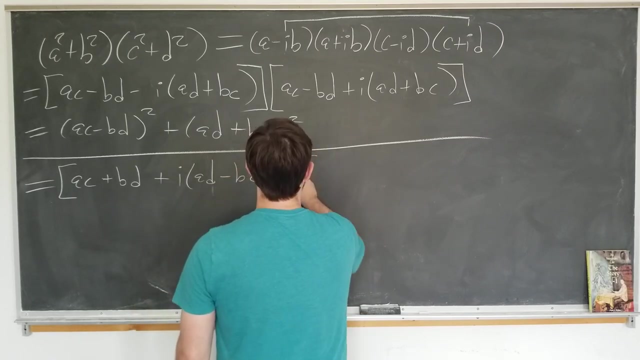 So it's going to be plus IAD, minus BC. I'm choosing the convention of putting the A's and the D's first. All right, This is our first term, And for the second term we're going to multiply the inner terms. 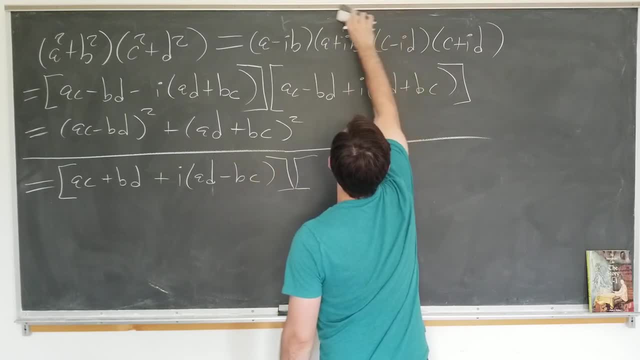 We did the outer term, Now we're going to do the inner terms. All right, These brackets look terrible. I do apologize. All right, So this one is AC. The real term is minus. I squared BD, which is plus BD. 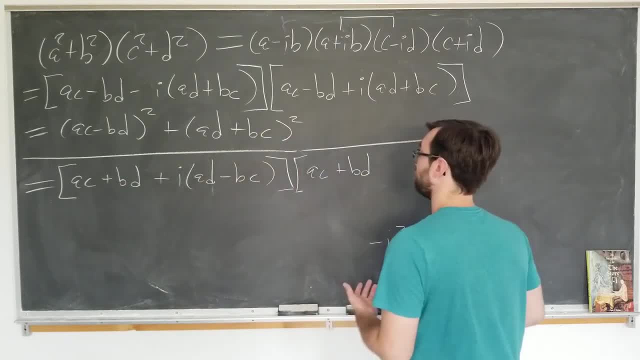 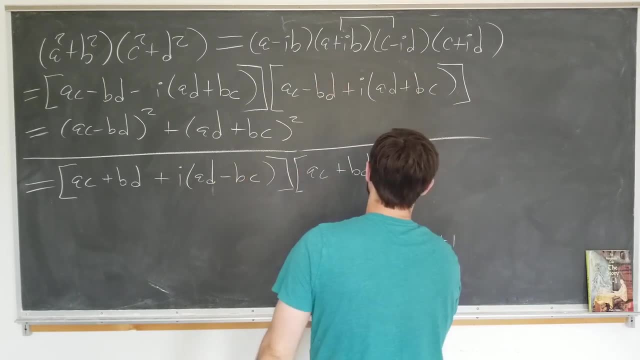 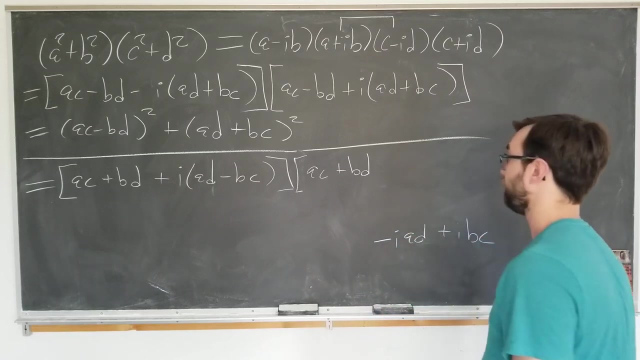 Great, We see. We see that it's the same for the real term And we would really hope that it's minus. I times that here. So let's see if it is The imaginary term minus IAD, plus IBC, which is exactly what we want. 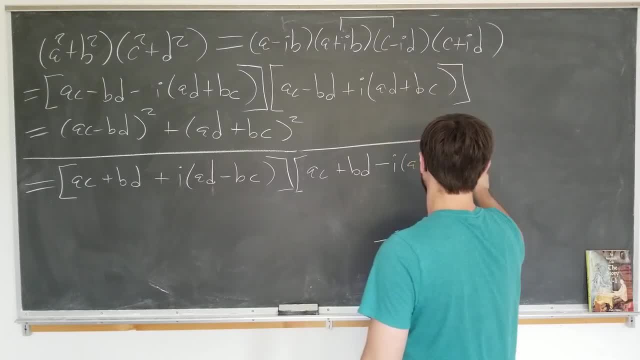 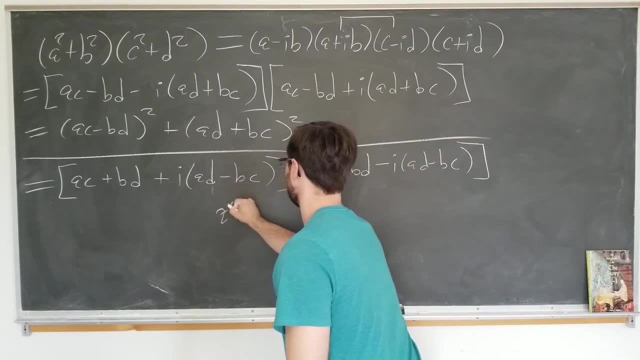 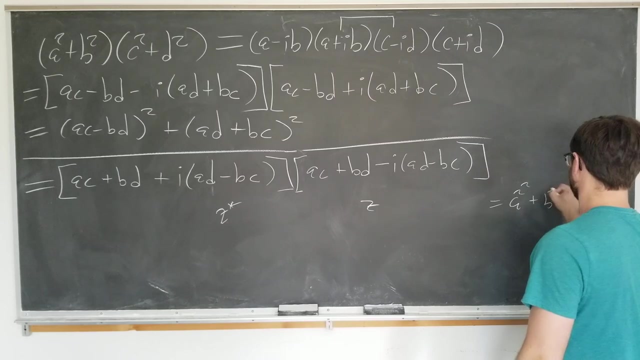 So minus IAD, minus BC. Now we can use the same observation as before and immediately write this as a Z star, Z Style number. So it's sum A squared plus B squared, Which we can do now Very easily to obtain our second solution. 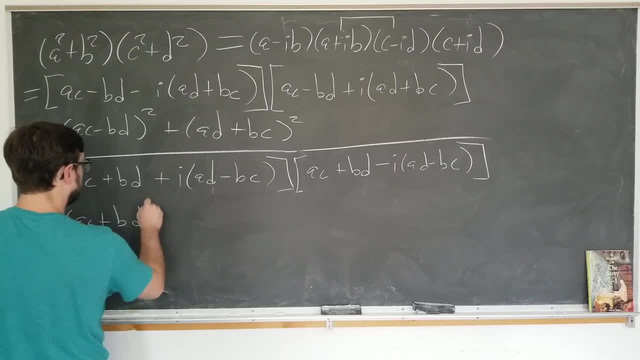 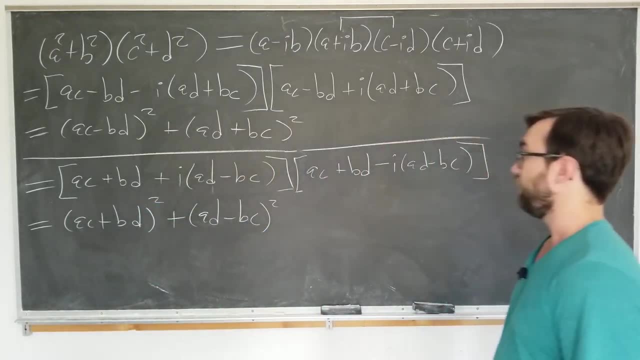 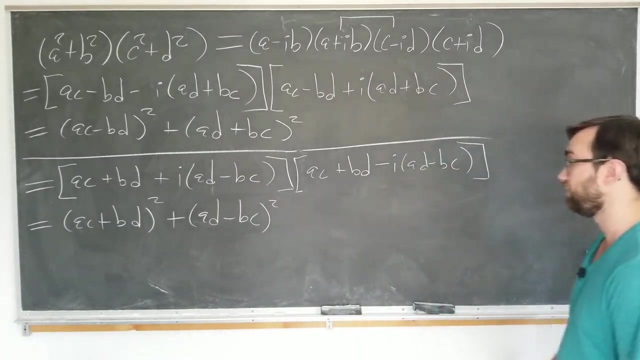 It's just AC plus BD squared, plus AD minus BC squared. Yeah, So, as you note, it's just what we had up above, But with the plus and the minus And it's not interchanged, which makes kind of intuitive sense. 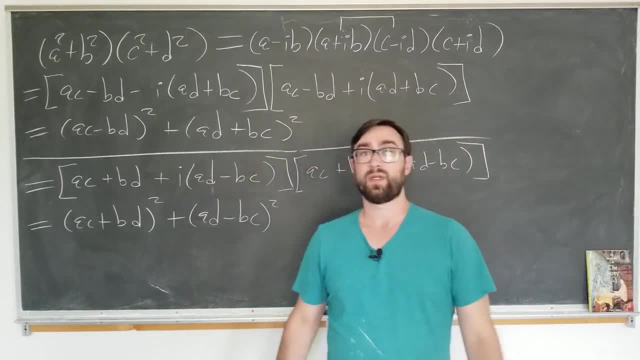 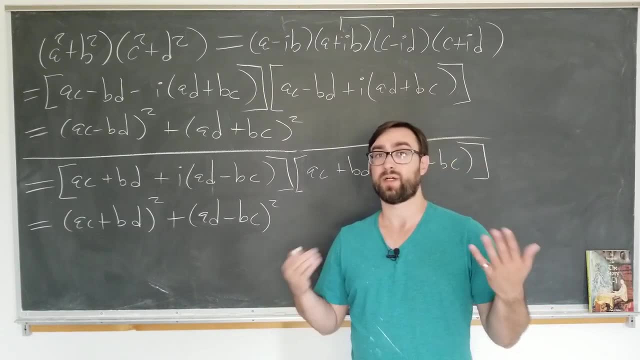 So now I have completed the proof. I've told you that there are two ways you can do this, And I haven't really showed that there are only two ways. I don't actually know how to do that. If you do, please leave a comment. 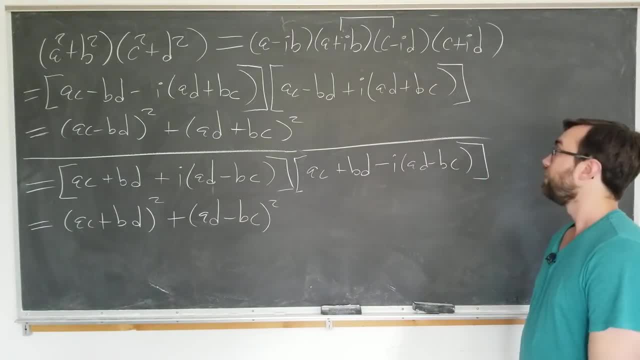 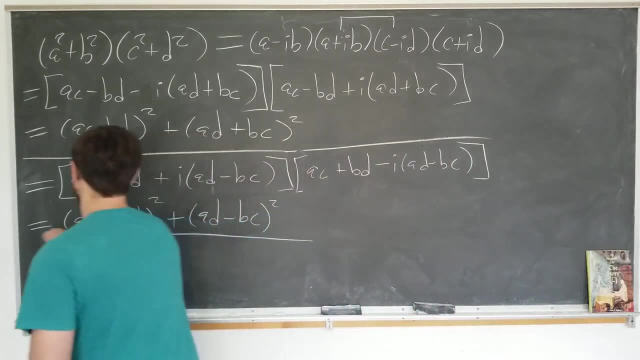 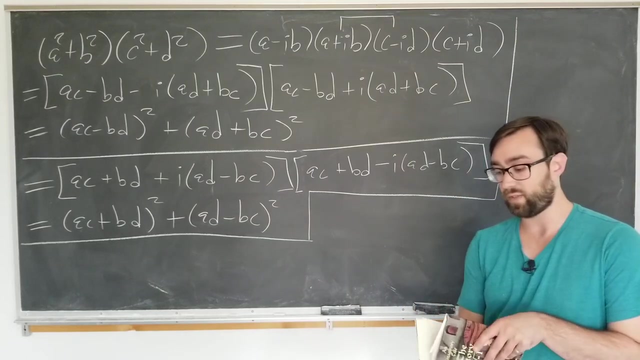 But there are at least two ways. There could be more, But why have I done this? What is the good of doing this if we don't actually use it for something? Well, let's go ahead And, as the book Indicates, let's use it to find the solution for our original problem. 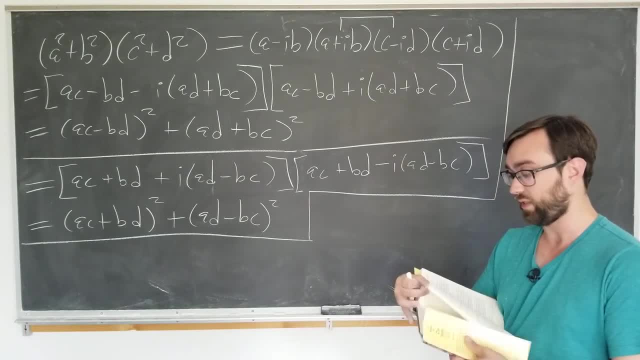 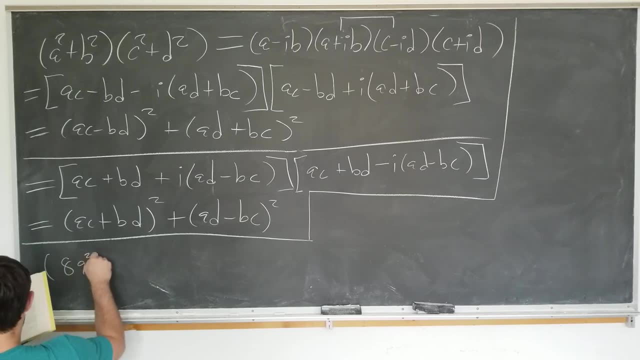 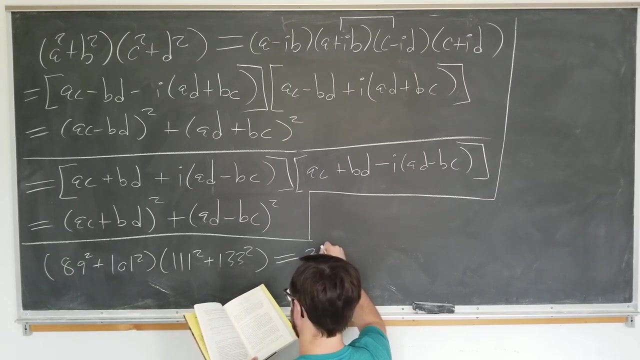 So if we plugged in ABC and D to this expression, we could indeed find the following: That 89 squared plus 101 squared times 111 squared plus 133 squared is actually equal to 3,554 squared plus 23,048 squared. 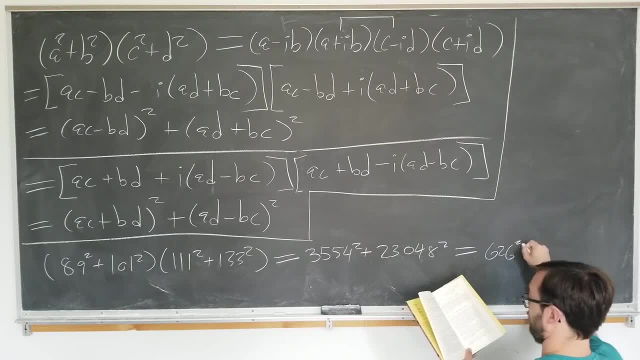 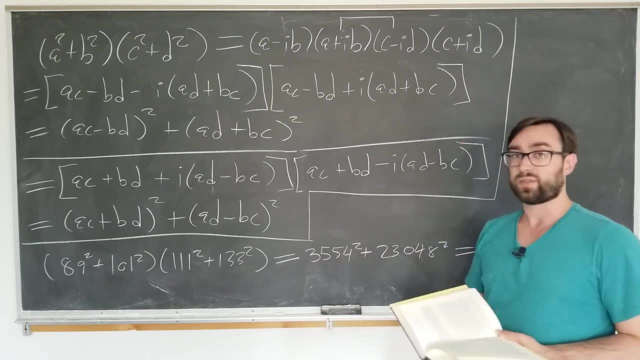 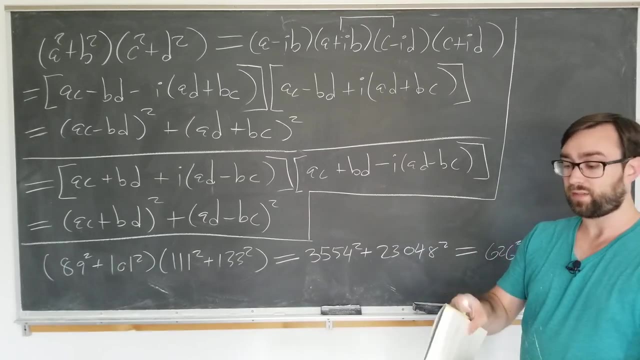 which is also equal to 626 squared plus 23,312 squared. If you want to, you can certainly square this all out, But I'm just going to trust Mr Nahin on this. So yeah, that's how you can use this. 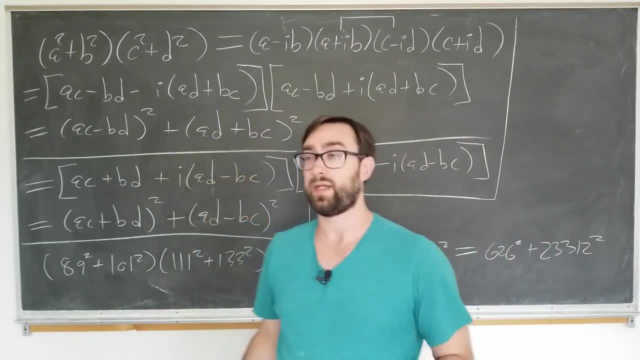 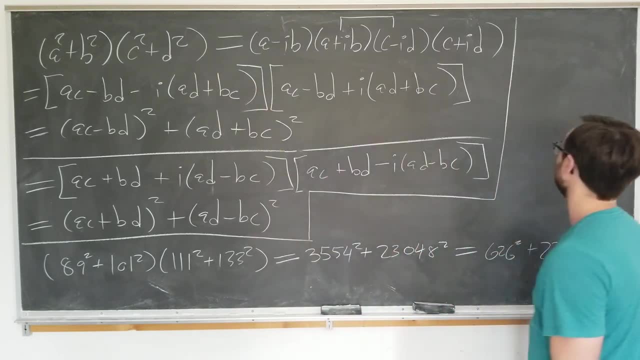 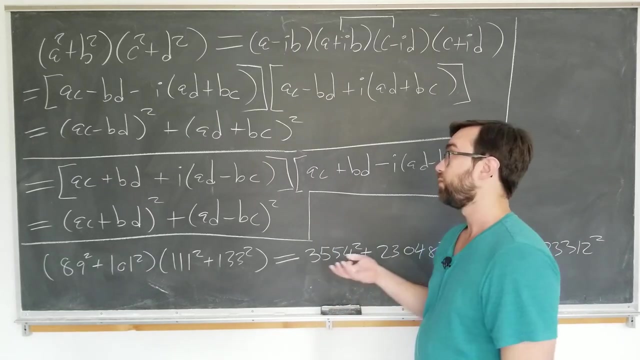 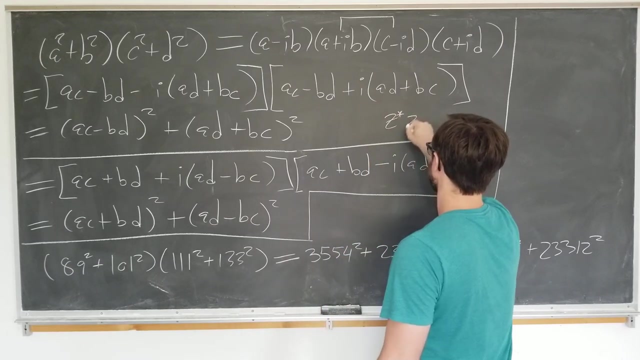 To find the U1 and the U1 and 2, the V1 and 2. If you're given ABCD squared in this kind of way. But the real question that I had while working through the proof is: why does this combination magically have a Z star Z style where everything just works out nicely? 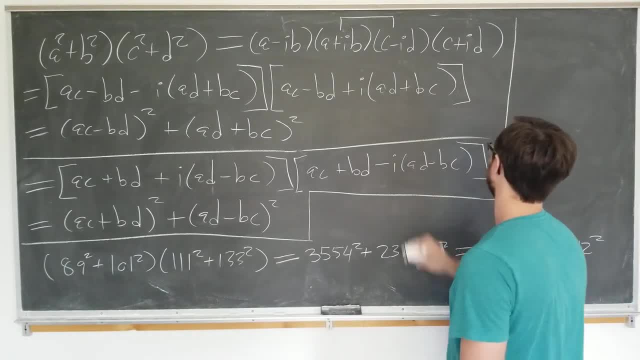 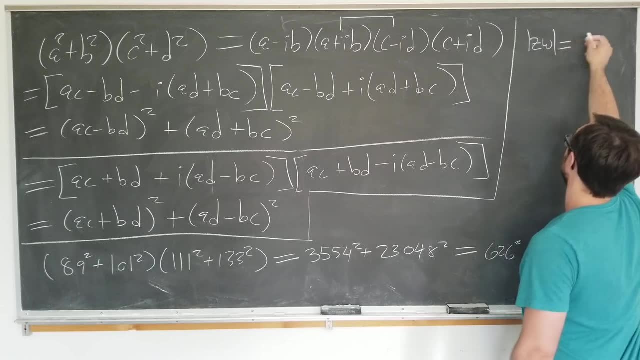 Well, it's actually A consequence of two simple rules. If we have two complex numbers- Z and W, and take the magnitude of them, it's the same as magnitude of Z times magnitude of W. And also the magnitude of the conjugate is the same thing as the magnitude of the complex number itself. 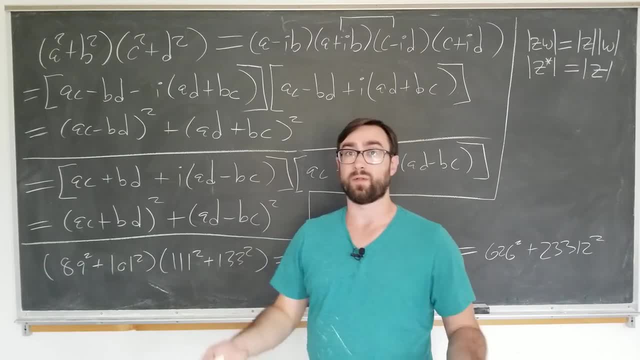 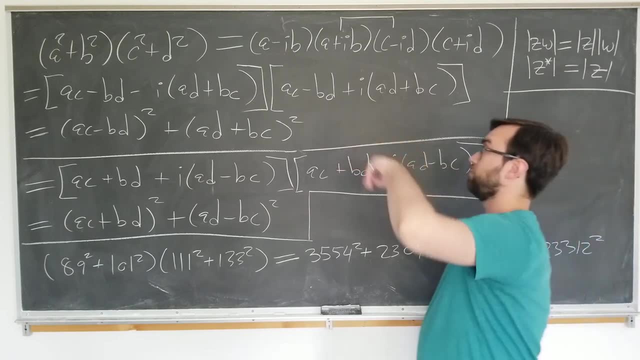 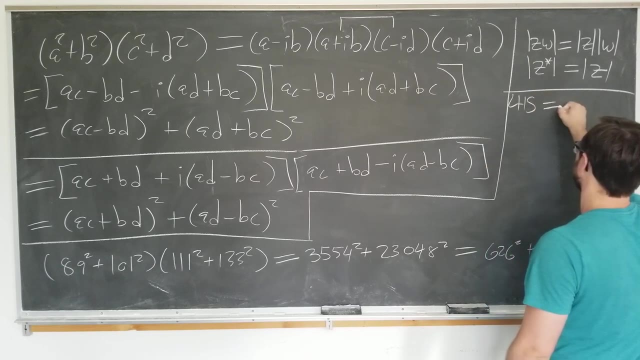 I want to go through the proof that we did here in a more general method to illustrate this. So we're going to do it as follows: We're going to look at what we had here, immediately recognize it as a modulus squared, So left-hand side of our expression. here is just Z star, Z W, star W.